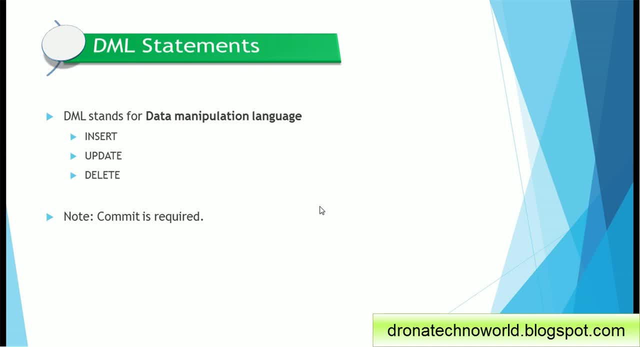 transaction in upcoming session. But we have to remember that if you are using any DML statement, we have to explicitly use the commit statement. Of course we can configure the statement, We can configure the statement and we can configure the tool to do the autocommit, But it is good idea to do the manual. 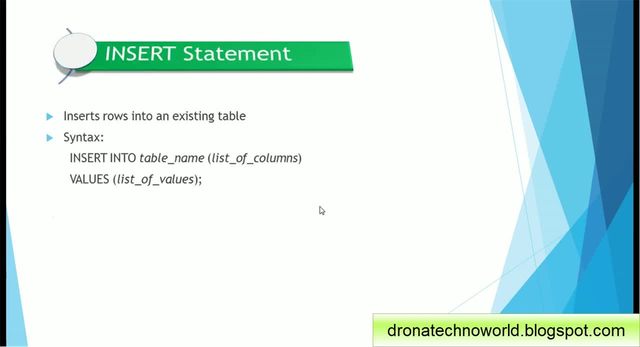 commit as a safer side Insert statement. as I said, it inserts the rows into, into an existing table. The syntax is very simple. We have to use keys such as insert into. Those are the keywords we have to use. After that we have to use: 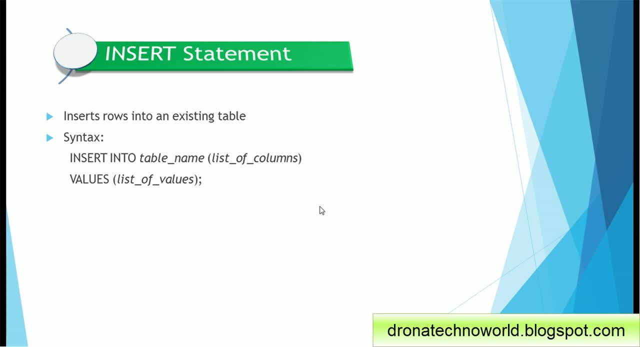 the table name, Then we can give the list of columns which we want to insert and then you have to use keys to insert the columns. So we have to insert the columns, We use keyword called values and then in the simple bracket we have to provide: 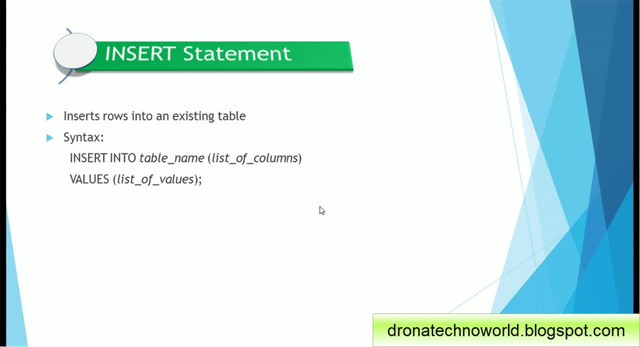 the list of values which we want to insert in the list of columns which we are going to provide. It's very simple. We'll see the demo on it very shortly. We'll also see what will happen if you do not pass the values or if you. 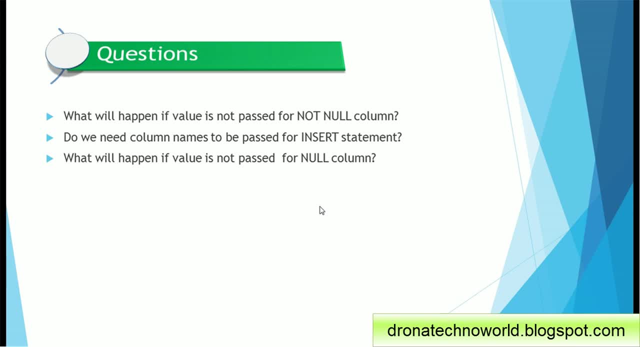 pass the values. if you do not pass the values for the not null column, We'll see what will happen. if the list of columns which we provide in the column list here, if you see after the table name we have to provide the column list, What will? 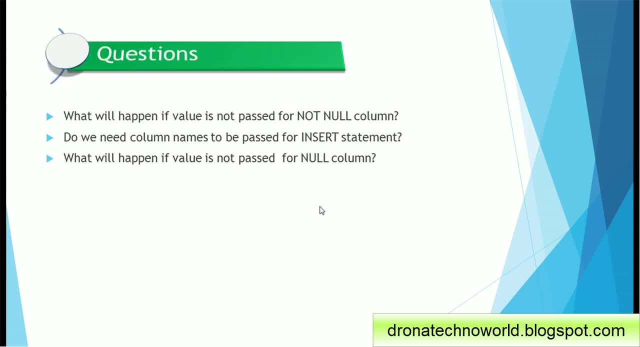 happen if you do not provide all the columns in that list. We'll also see if the list of column which we are providing, if it is a nullable column and if you do not provide the value, what will happen in that particular column. So there are some interesting things. 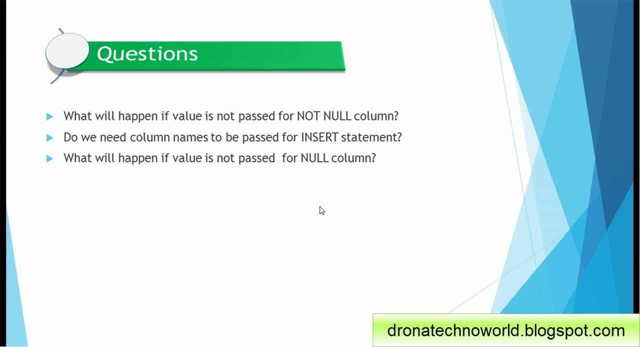 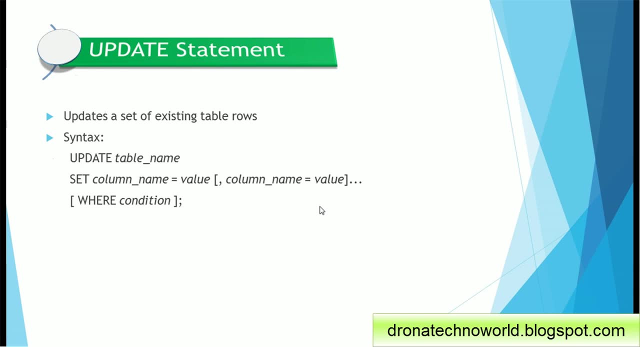 and we'll see that in our demo also, and we'll get the answers to that- those these questions during the demo. Update statement. Update statement is used to update a single record or multiple records in the existing table. The syntax is very simple. You can see here: 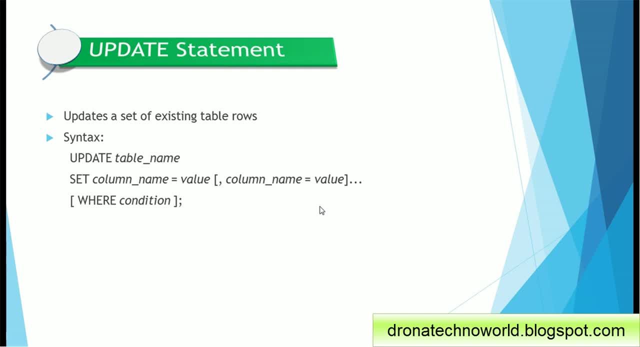 we are to use a keyword, update space- and then use the table name which we are going to update here, to use the set as a command to update particular column. So after set, we are to provide column name equal to sign and the value, If you have the multiple columns update. 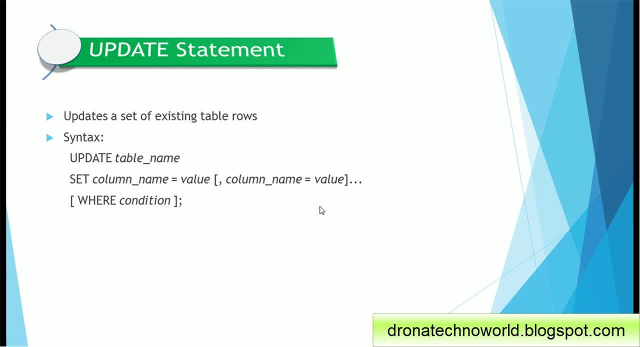 then after the first value, then we can use a comma, then the second column name and the value which we want to update to that column and then optional where clause we can use. means if you do not use the where clause, whole data set will be updated. 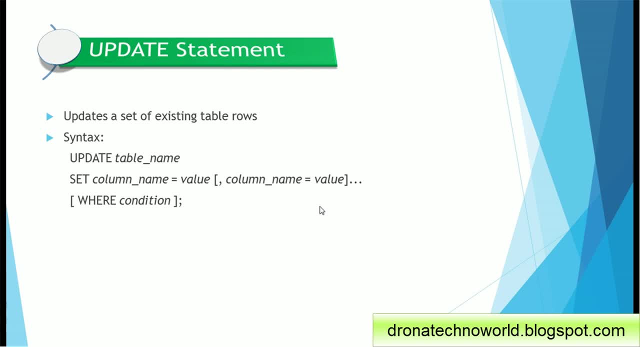 If you use the where clause, the filter or the conditional values will be updated: Delete- Delete is very simple, It's very straightforward. Delete from table name, So delete from. these are the keywords, and then we have to use the table name. Of course we have the where condition. 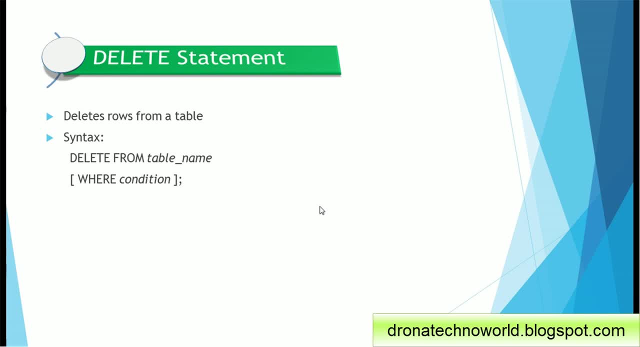 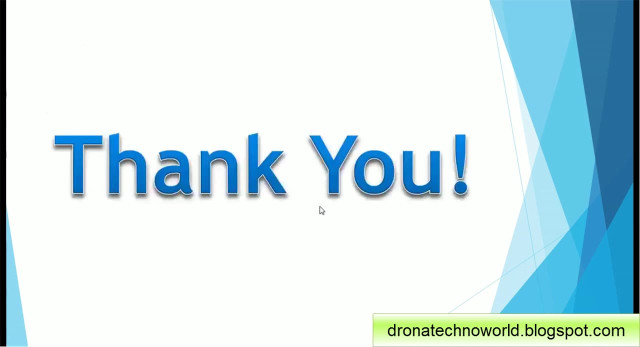 also, which is optional, If you do not use where condition, then whole data set will be deleted from the table. If you want to delete specific columns Or specific rows, then we have to use the where condition. So these are the DML statements. 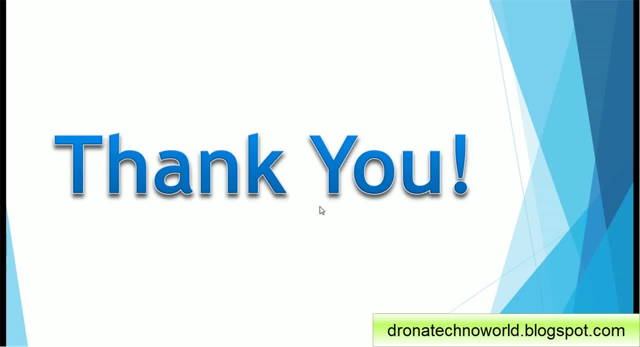 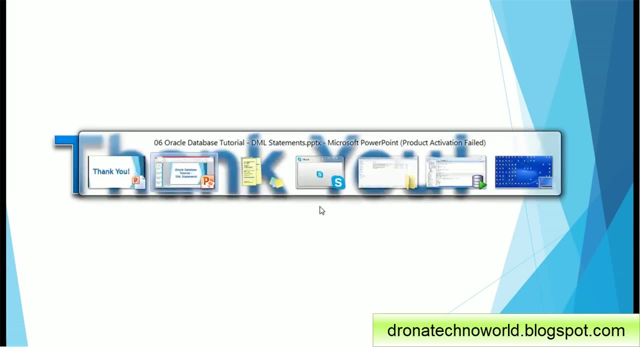 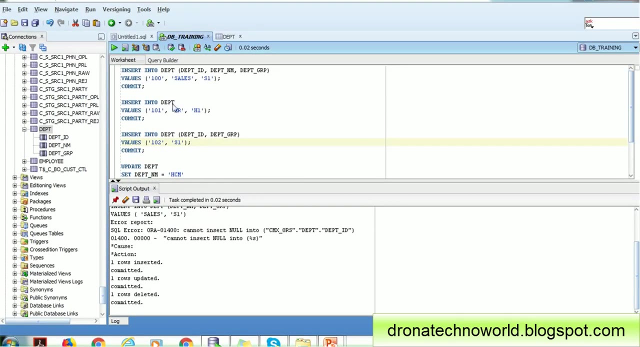 I hope you got this. I'm repeating again these are: there are three types of DML: insert, update and delete. Let's go back and have a demo on this items. So very first thing we are going to see is how to insert the data. 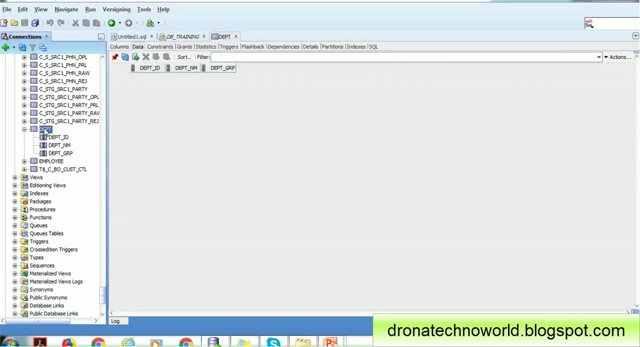 So you can see we have created a table. Sorry, we have created a table called department DEPT. DEPT has three columns: DEPT ID, DEPT name and DEPT group. that is, department ID, department name and department group respectively. If you see the column definition, all these are the where char 20.. 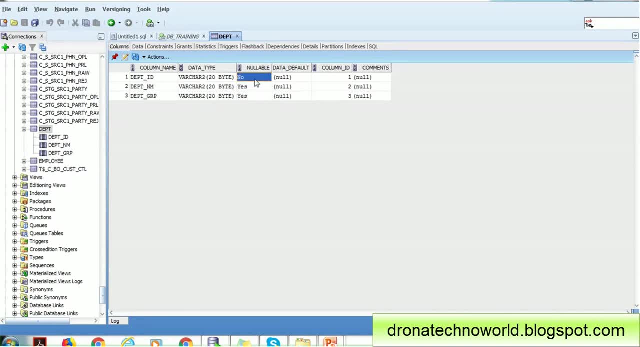 But if you notice, department ID is not nullable column. The rest of two columns, That is, department name and department group, They are nullable column. Just, I'm explaining this because in the demo we are going to use this column accordingly. Now what we'll do. 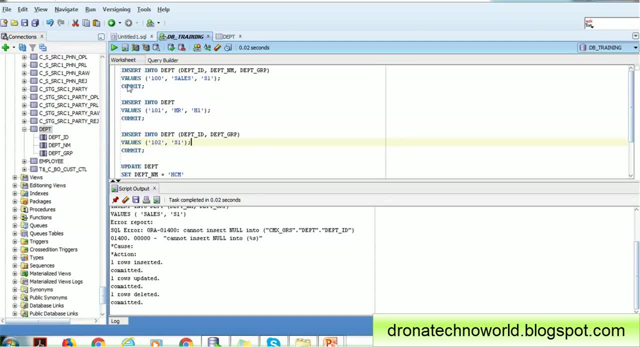 We'll insert the record in this table. The syntax is very simple. Let me clear up. Insert into table name that is DEPT, Then simple open bracket. provide the column name, such as department ID, department name, department group and the values we have to provide. 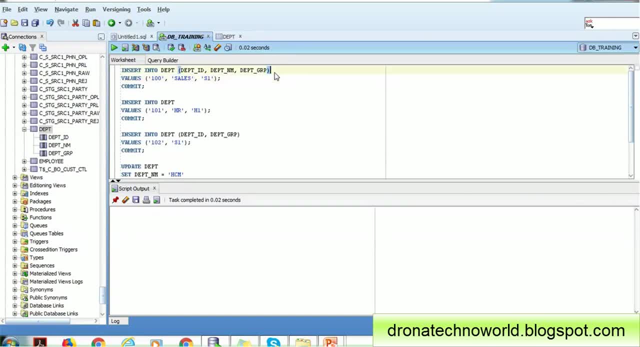 Make sure here we are not using any comma or semi comma after the column name. You just we have to use the space or go to the next line and type the values: open bracket. open, simple bracket. close, simple bracket and forward the values for each column. 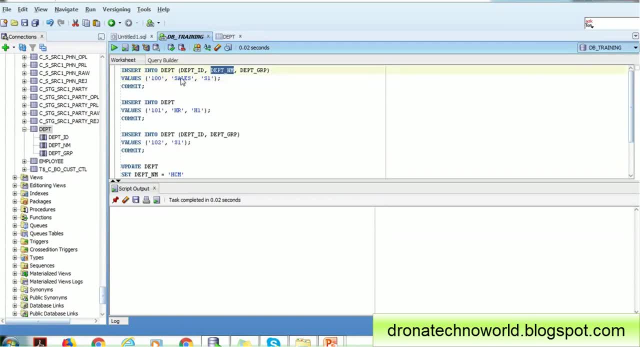 So department ID will be 100. department name will be the cells. department group will be S1.. You can give any values because it's a where char If you notice the values when you repass the values. if it is a where char we have to use. 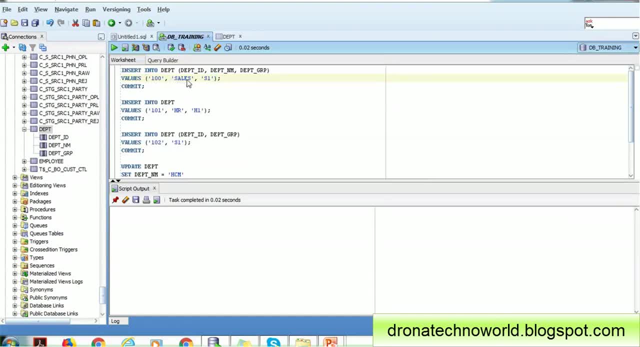 a single quote. Here you can see the next value and the first values should be separated by comma. So if there are multiple values we have to separate by the comma. At the end of this statement we have to use this comma. Sorry, semi comma. 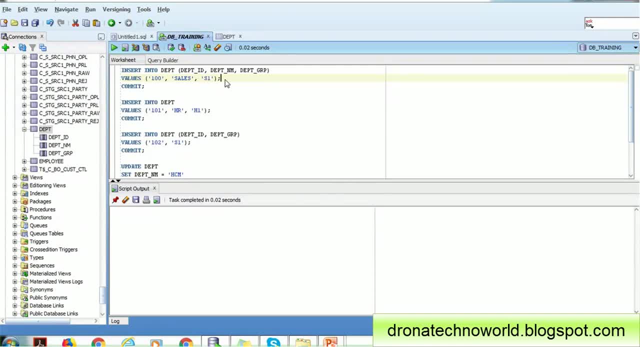 Semi comma. it tells the program- oracle program- it is the end of executable statement. Hence it is always recommended to use a comma after writing any executable statement. After that, as I said, commit is required to data. is the data which we are updating through DML get firmly or the finally stored in the database. 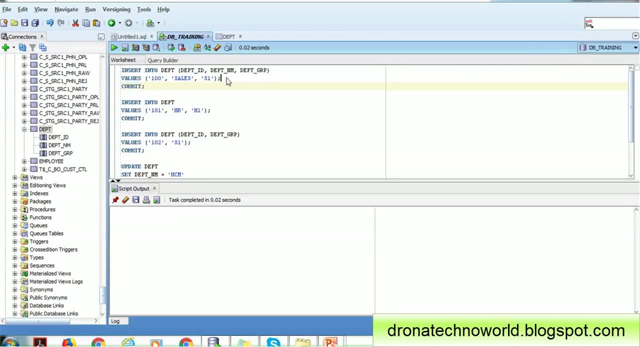 So commit is required. So I'll just Report this statement, select it and here are the two things. you can see the green arrow. it will execute. But on the right hand side of this green arrow there is a run script which will give us the 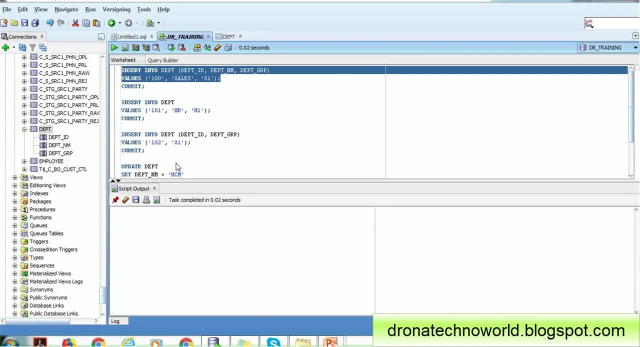 execution process. also here you can. on the console you can see whether it's executed or not. So let me execute using run script. Now you can see one row inserted If you want to verify that, but we have to make sure it's commit is done. 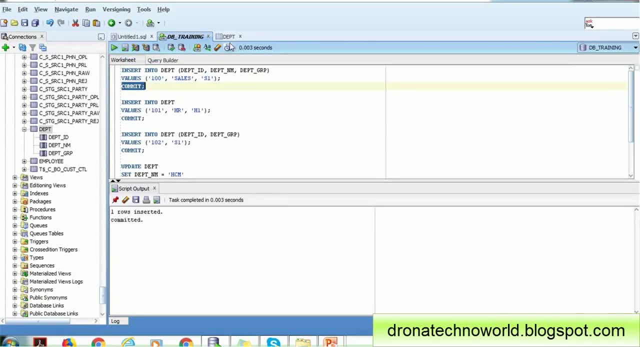 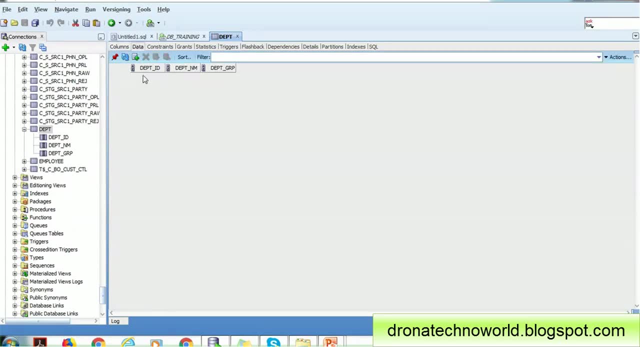 Select commit committed. If you want to verify, go to this table and there is a data tab. go to the data tab. You can't see anywhere because this table I already open, so you have to just refresh it here. if the data is committed properly, you can see the data here. 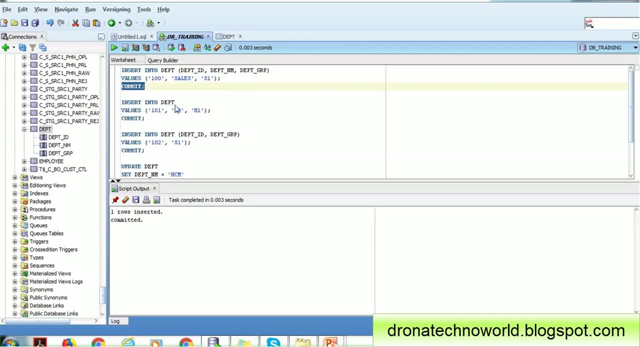 So this is the way we can use the commit statement. Now there is another way of insert statement. if you are inserting values for all column, like here, We have three column: department ID, department name and group by department group. If you are passing the values for all three columns, then we don't have to use the list. 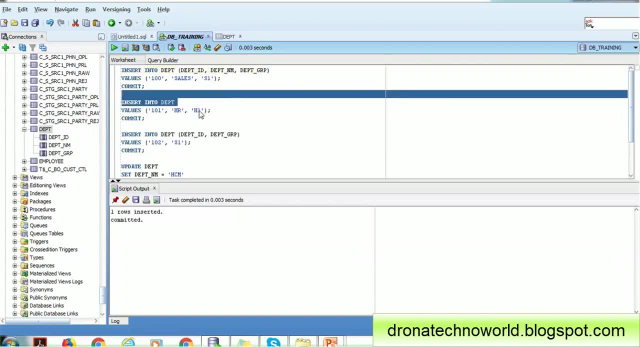 of columns. So I completely remove that list so you can just use insert into department DEPT and just pass the values and commit it. So I'm just using this and execute script so I can see one record is inserted and committed. So that means if you are passing all values, no need to provide the column name. 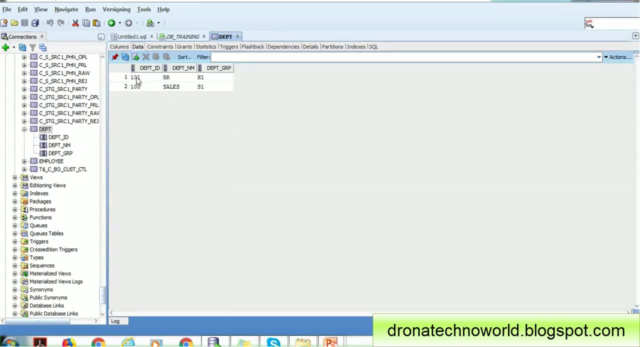 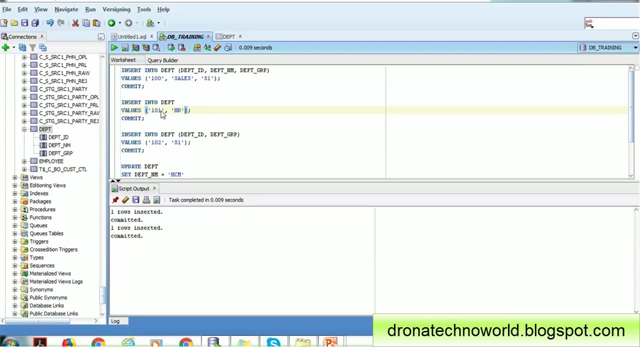 If you want to verify, just go here and refresh. I can see this column is added. Now suppose if you remove one of the column value, let me do something here and let's try to run here. I'll just use one statement here for now and execute it. 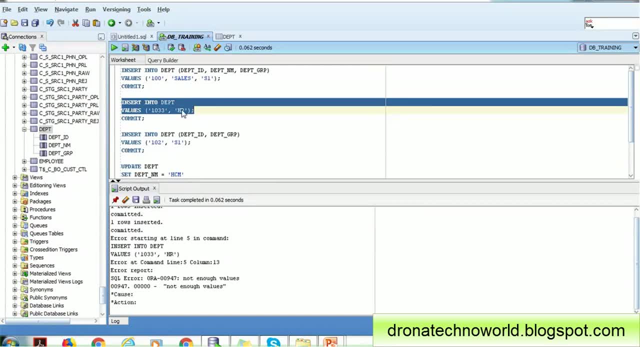 So if you do not pass all the values, Then it is mandatory to provide the column name. So for example, here I will execute the same statement, but this time I will not pass the group name. If you are passing list values, then it is mandatory to provide the column name or list. 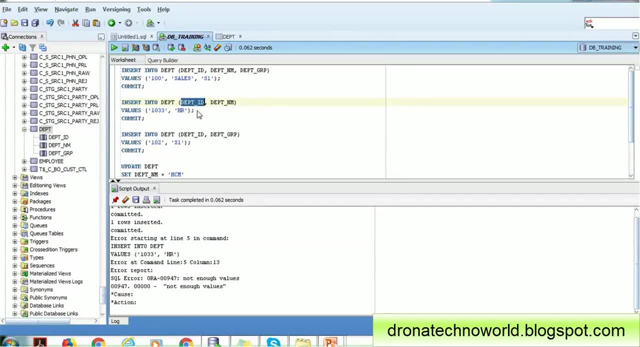 of columns. If you are passing all values, it is not mandatory to provide the column names, So I'll just reuse now And execute. Now, one row is inserted. The next thing we are going to say is what will happen if you do not provide a column. 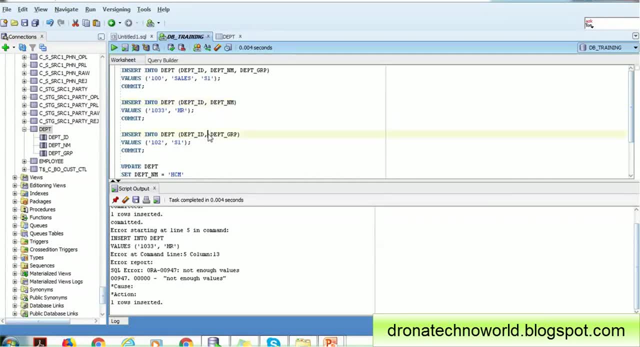 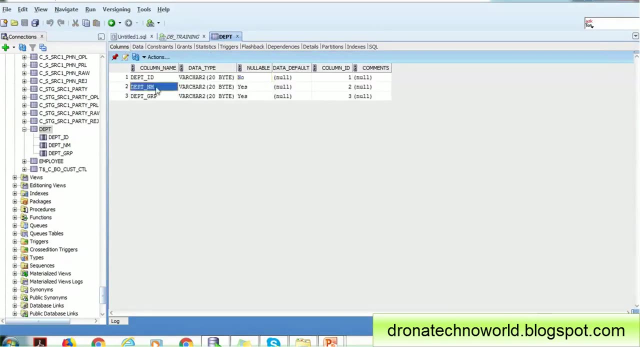 name. For example, if you do not provide column name here, which is a department name, I'm just passing department ID and group ID Here. the department name is nullable column If you see here The department name is nullable column. So what will happen? we'll see in this example. 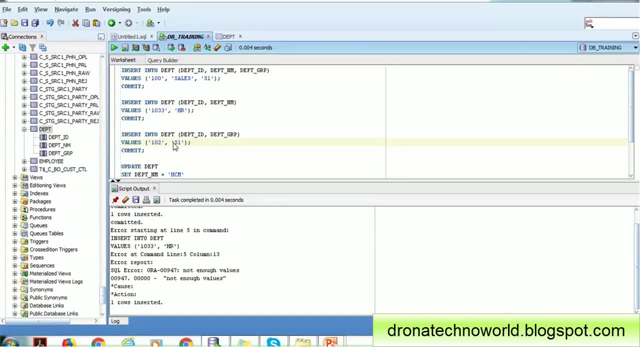 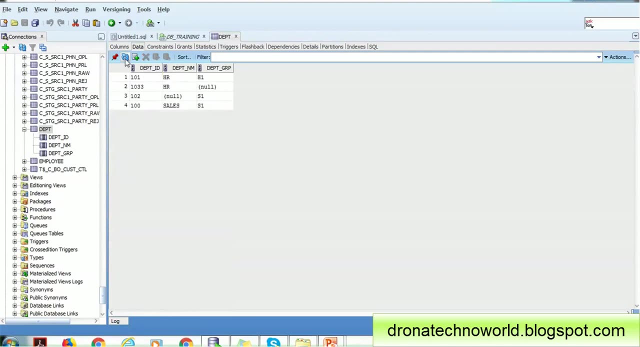 I'm passing the department ID as 102.. Department group as S1.. Just execute it Here. I can see one row is inserted and commit has happened. So I'll go and see whether 102 is inserted or not. Yes, 102 is inserted and under the department name. 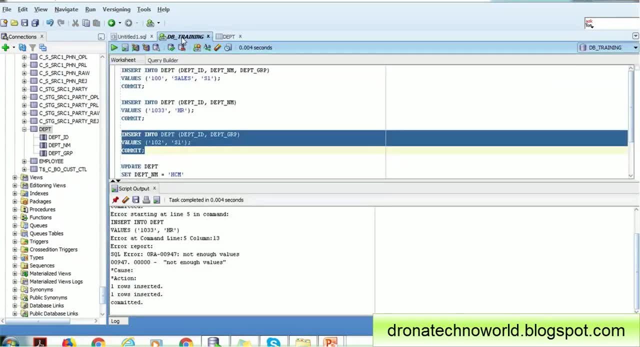 I can see the value null is inserted. So if it is a nullable column and if you do not provide the value, the null values will be inserted. So I'll just do here first department name and let me pass some value here. this time I will not provide. 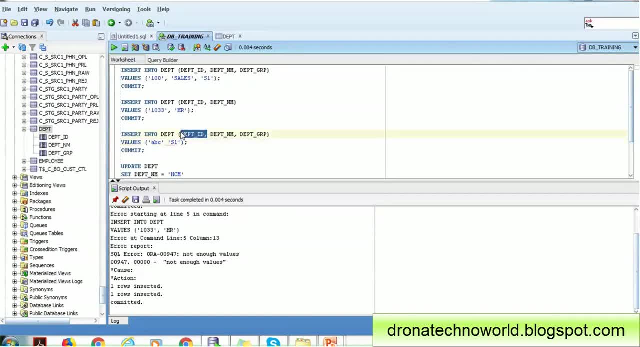 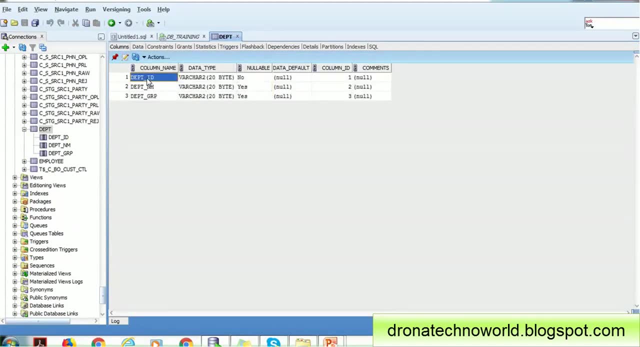 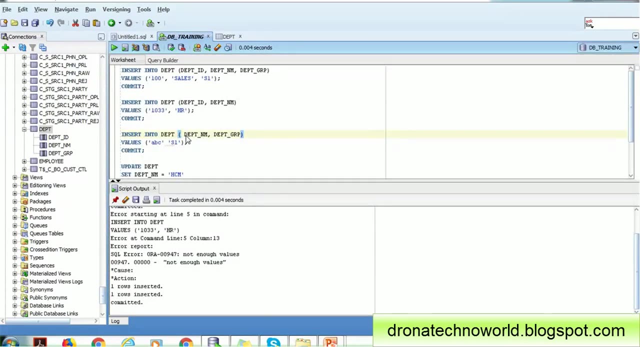 Let's see what will happen if you do not. before executing this statement, let me show you one of the thing. So if you see here, department ID is not nullable, If you do not provide a value to not nullable field, what will happen? We provided department name, we provided the group name- group, department group- and let's 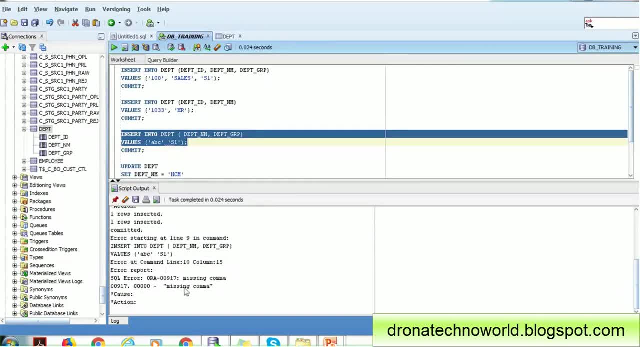 execute it. So it is showing the error message. it says some 00917 or 00917.. So it is misleading message, though it's like it says missing comma, but actually it is mandate. okay, so let me see here we are missing comma. let me execute again. clear it. 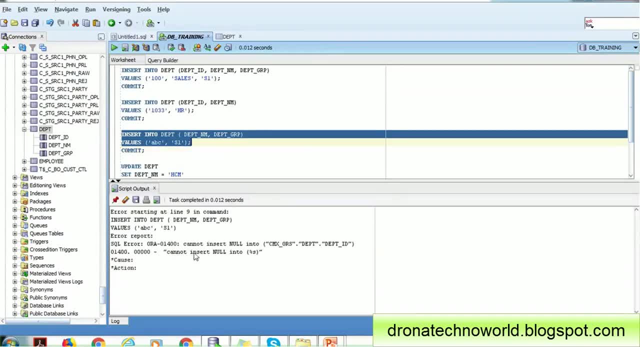 Now execute. Now it will give the message: Aura0144 cannot insert null into department ID. The reason is: department ID is not null and if you do not pass value, it passes the null value. Hence it will throw the message saying that cannot pass the null value to the department. 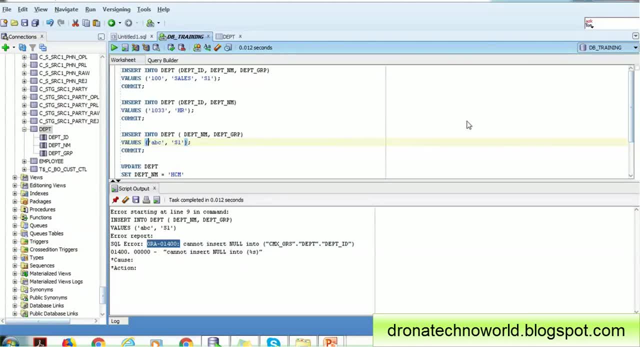 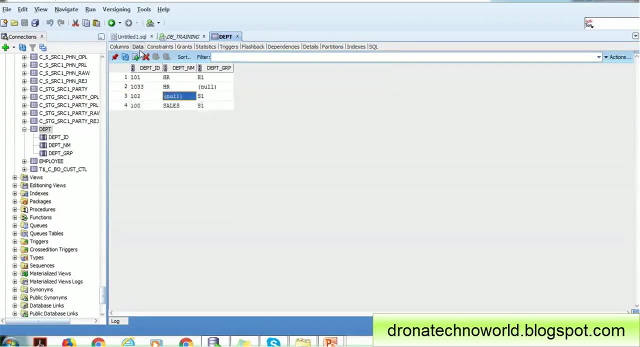 ID. We can pass the null value to nullable column, but not to the not null column. Now the department ID is not null Now. it is not null Now. if we pass the message Now, let's try to use the update statement. 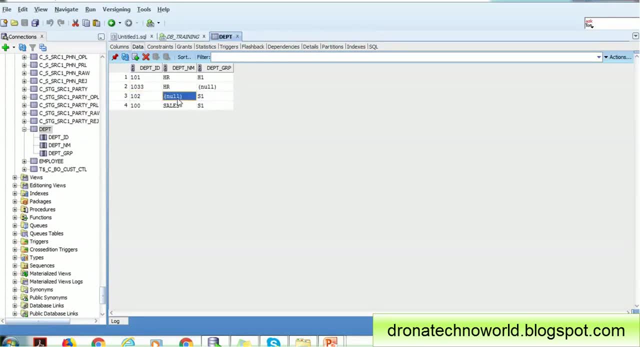 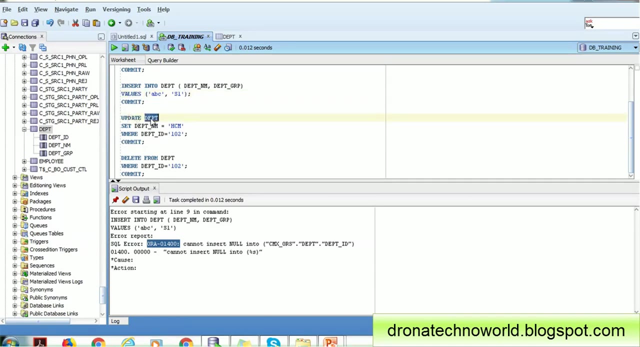 By using update statement, we will try to update the department name. So we will get this department ID 102, because this is unique in this column, So we will use it 102 and update this department name. Let's try that What we are going to do. we are going to update a department. 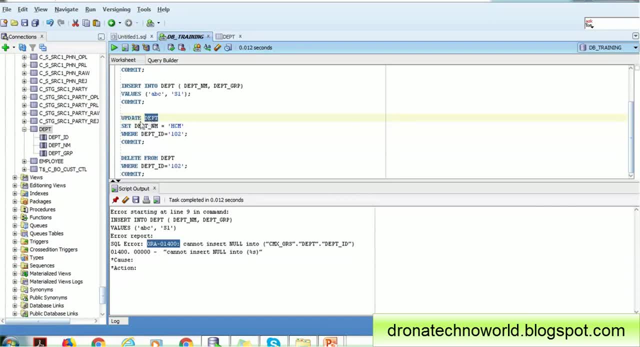 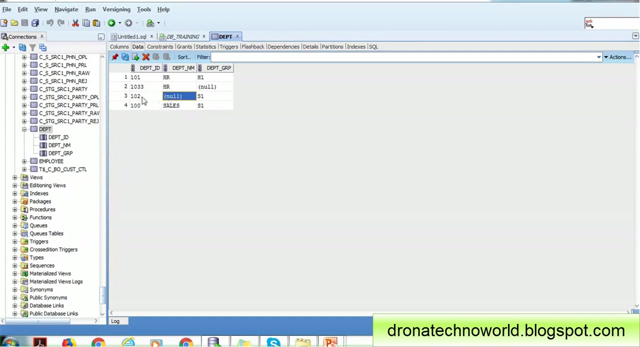 So syntax is update. then table name values, set department name. you can pass any value. I'm passing HCM and we are using where clause, So where clause, department ID equal to 102.. So it will. it should update the department name to HCM, where the department ID is 102. 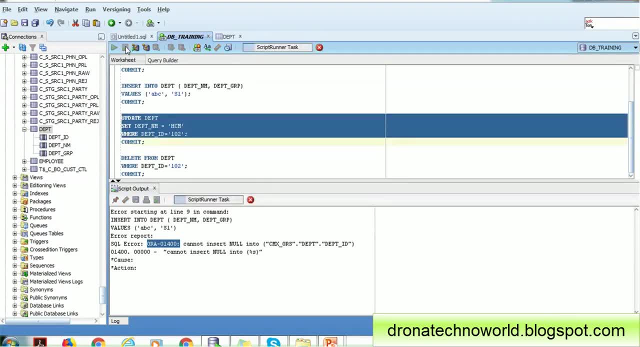 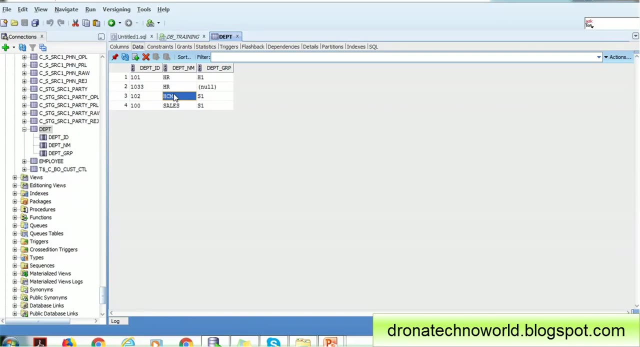 So let's run it. Okay, I just executed it. I can see one row is updated. Let's commit it Committed And we'll see here the data. Just did refresh. Now I can see the department name is populated as HCM, corresponding to department ID 102.. 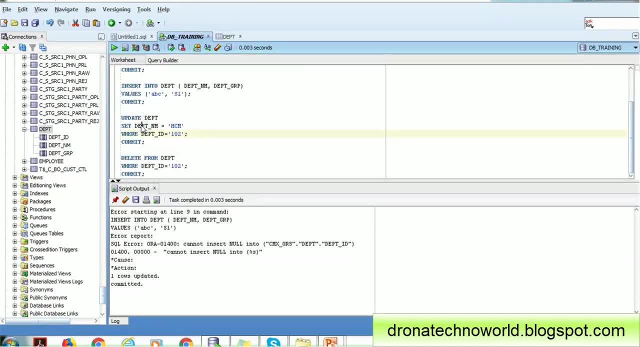 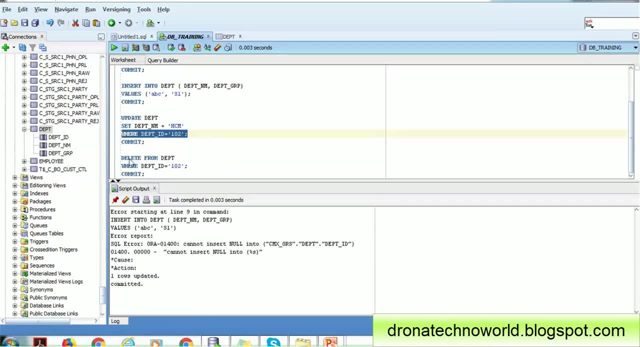 Update, Update, Update, Update. Let's try to use the delete statement. In order to use the delete statement, syntax is delete. from then we have to use the table name, that is, department DEPT and where clause department ID 102..